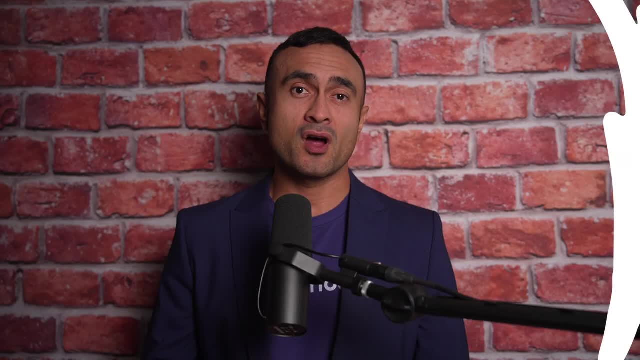 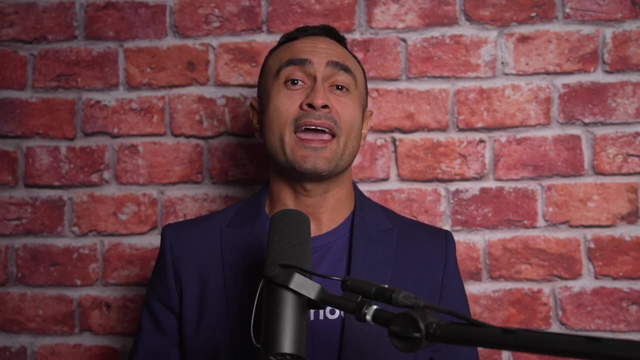 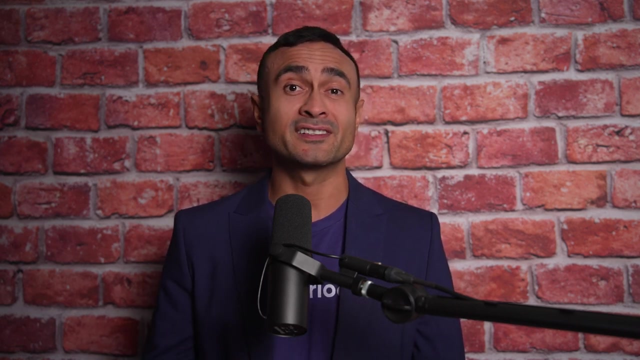 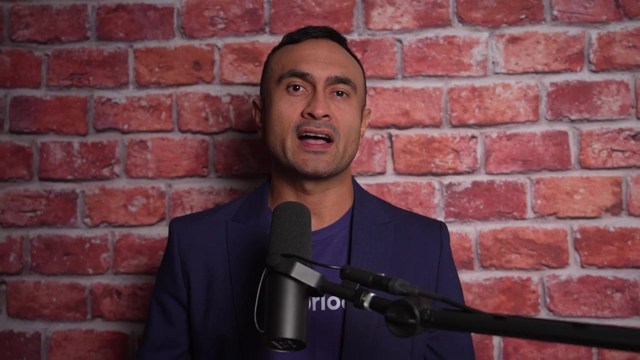 Automated Property Valuation. Automating the valuation process saves considerable time and effort for owners, Property management companies, real estate companies and other players in the real estate sector. In fact, automated property valuation removes the element of subjectivity from the process. Human biases, personal opinions and emotions can influence traditional valuations. 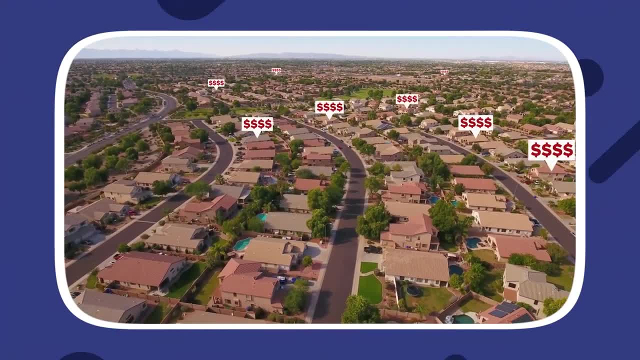 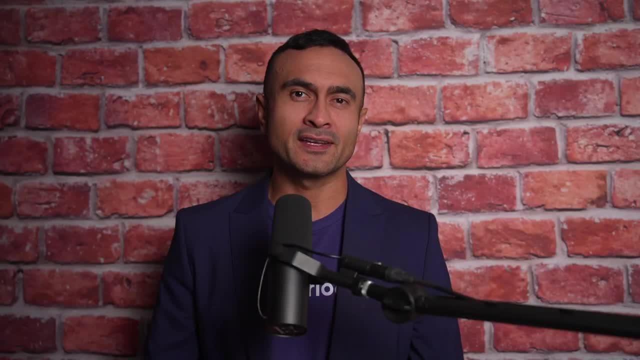 However, AI algorithms analyze data objectively, eliminating bias and providing you with an impartial assessment of a property's value. This objectivity empowers you to make strategic decisions based on data-driven insights rather than gut feelings. It helps you determine the right property value, whether you are looking to sell a property. 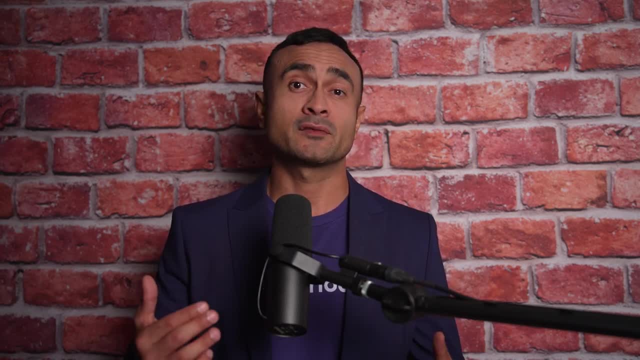 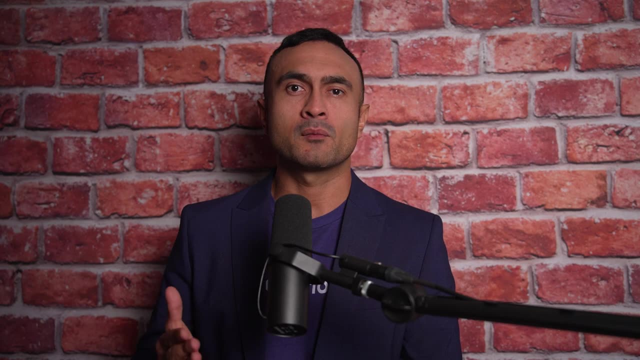 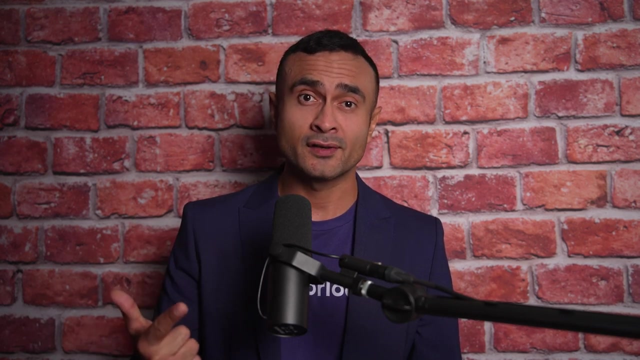 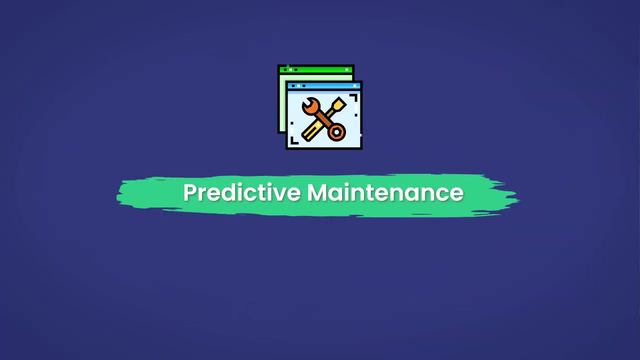 determine rental rates or evaluate potential investment opportunities. AI-powered valuations provide you with reliable estimates that align with current market conditions, so that you can optimize pricing strategies, make informed acquisition decisions and modify your property portfolio And stay ahead in the real estate industry. 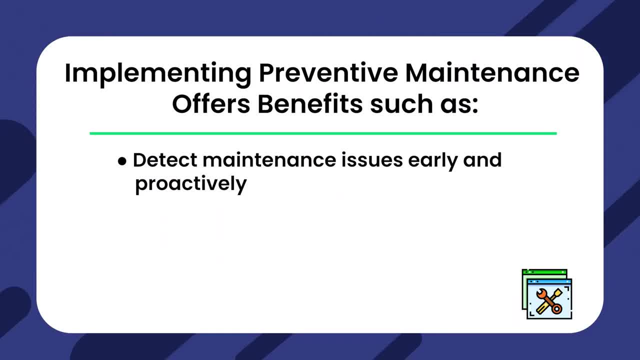 Predictive Maintenance. Implementing predictive maintenance offers benefits such as Detect maintenance issues early and proactively, Reduce tenant complaints and minimize disruptions, Optimize budget and resource allocation, Improve the efficiency of maintenance tasks, Enhance the lifespan of building systems and equipment, And much, much more. 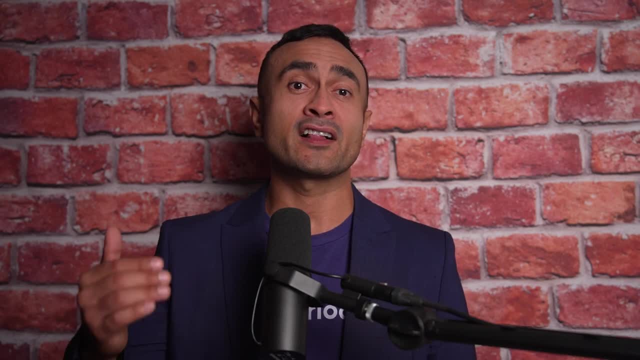 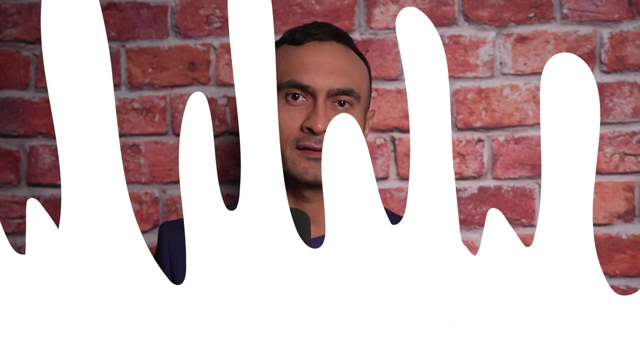 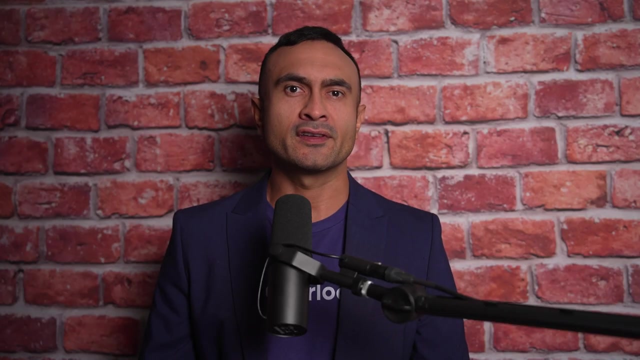 It's important to note that, while predictive maintenance is a valuable tool, it doesn't entirely eliminate the need for routine inspections and preventative maintenance. Regular inspections coupled with predictive maintenance create a comprehensive maintenance strategy that ensures the optimal performance and longevity of your building systems. 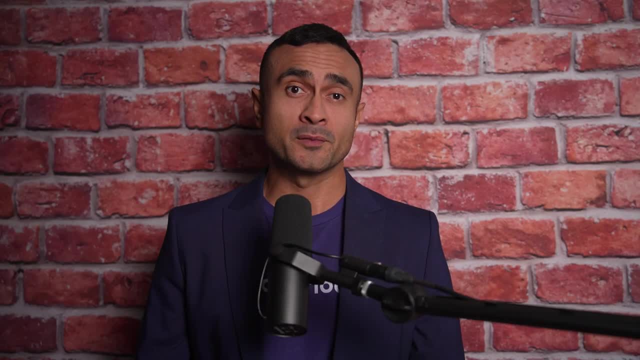 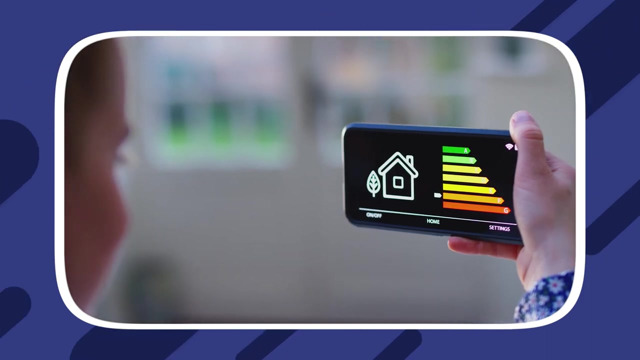 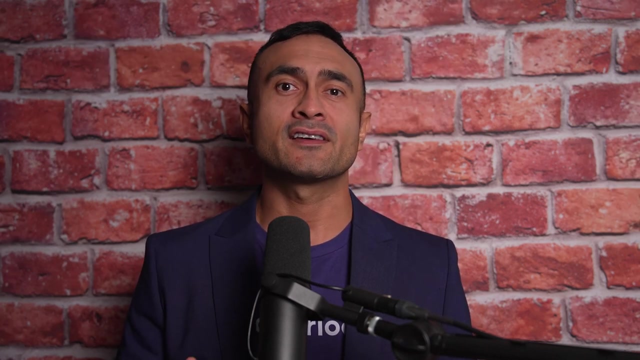 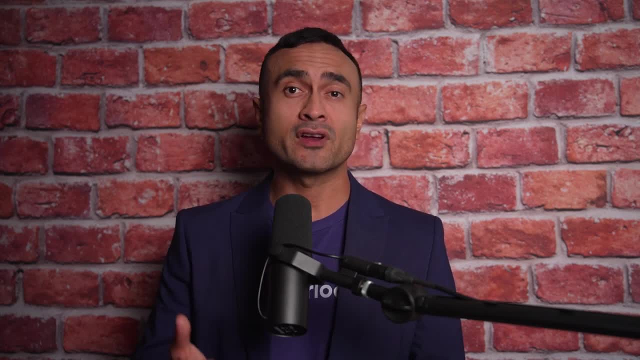 AI-powered smart energy management systems analyze vast amounts of data, including energy consumption patterns, occupancy rates and energy consumption patterns. AI-powered smart energy management systems analyze vast amounts of data, including energy consumption patterns, occupancy rates and energy consumption patterns. Power tools provide valuable insights and recommendations to help you enhance energy. 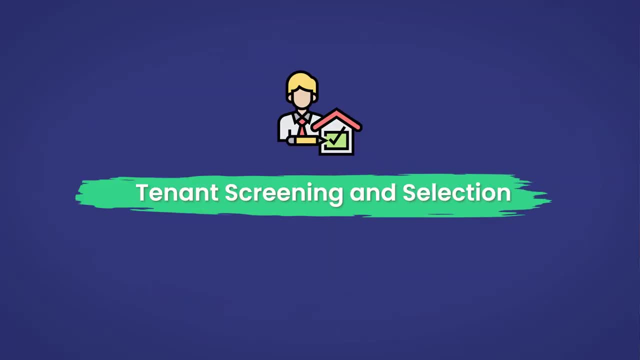 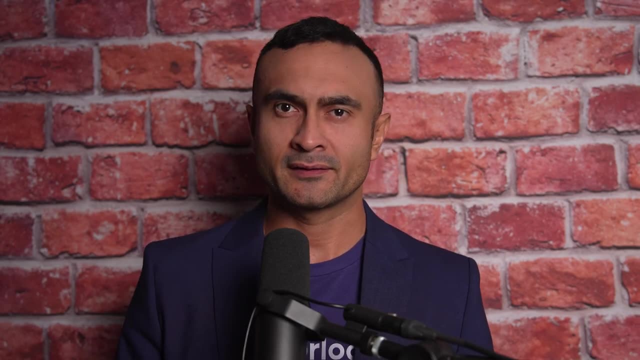 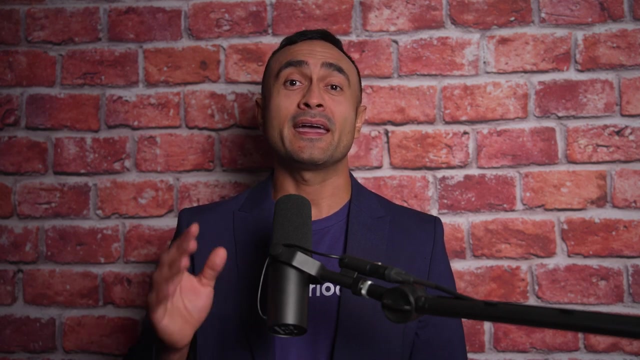 management and reduce your carbon footprint. Tenant Screening and Selection. Traditional tenant screening processes often involve manual evaluations and subjective decision-making, leaving room for human bias and potential risks. AI property management tools have changed this. AI-powered algorithms analyze potential tenants' credit history, employment records, rental. 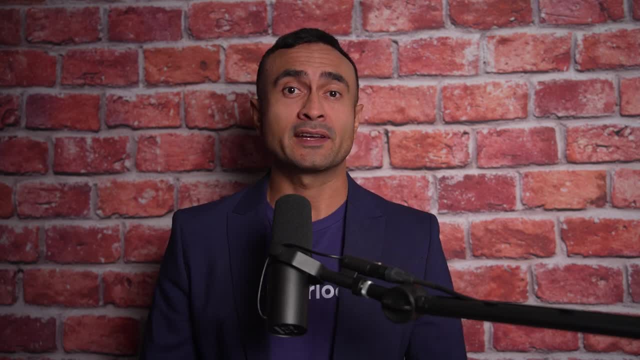 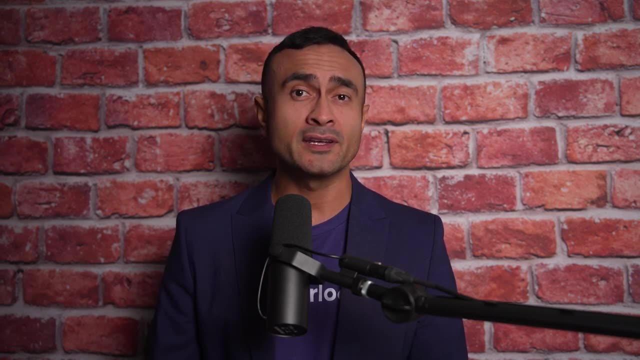 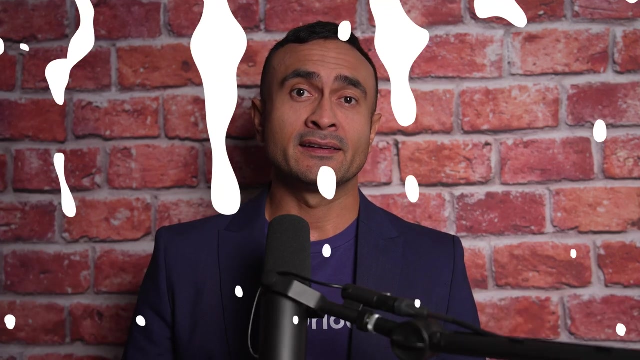 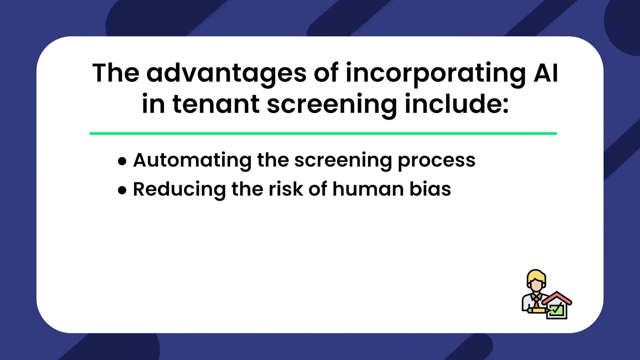 history and public records to evaluate prospective tenants objectively and efficiently and provide a comprehensive assessment of a tenant's reliability, financial stability and sustainability for your properties. The advantages of incorporating AI in tenant screening include automating the screening process. reducing the risk of human bias mitigates risks associated with prospective. 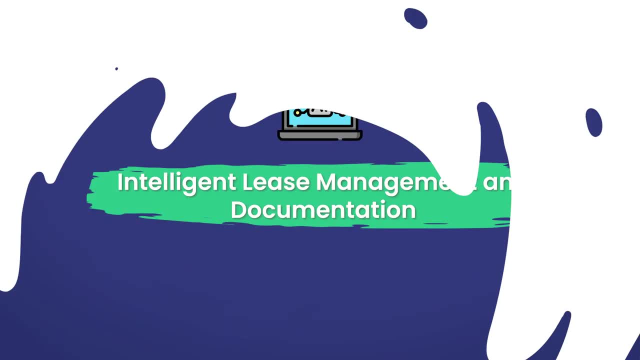 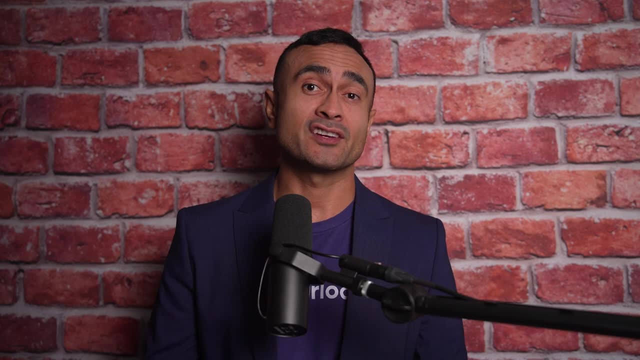 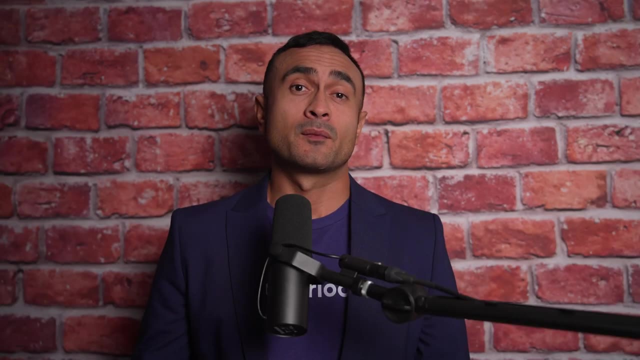 tenants, Intelligent Lease Management and Selection. Traditional tenant screening processes also provide a comprehensive assessment of a tenant's reliability, financial stability and sustainability for your properties. AI algorithms can create lease agreements by taking important details like tenant information and property specifications into account. AI can also calculate rent automatically, considering factors like rent increase clauses. 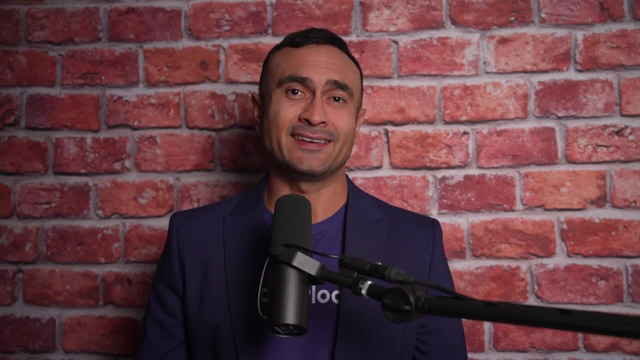 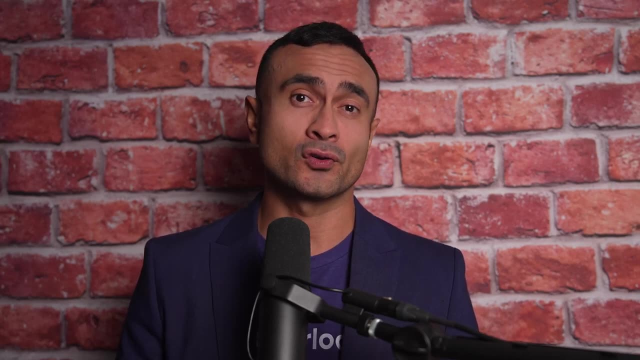 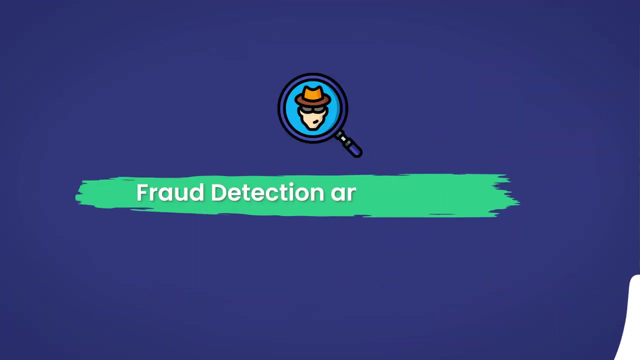 Property management software often uses AI to track lease dates and send reminders for renewals, reducing vacancies. AI also helps in organizing documents securely, eliminating the need for physical storage and making retrieval quick and easy when needed. Fraud Detection and Prevention: Unfortunately, the real estate industry is not immune to fraudulent activities. However, artificial intelligence provides property managers with advanced fraud detection and prevention systems to safeguard properties and investments. AI-powered fraud detection systems utilize sophisticated algorithms to analyze patterns, anomalies and deviations in financial transactions and activities. The AI-powered fraud detection systems utilize sophisticated algorithms to analyze patterns. 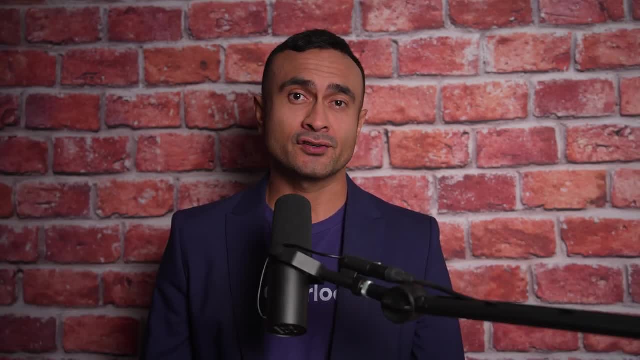 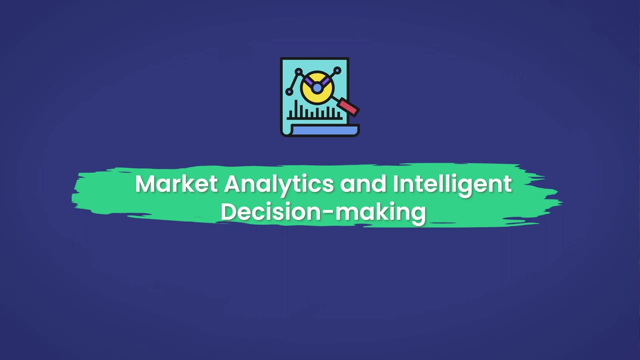 anomalies and deviations in financial transactions and activities. This is integral for early fraud detection, so that you can intervene in a timely manner and protect your investments. Market Analytics and Intelligent Decision Making: Staying informed about the real estate market is essential for making strategic decisions. 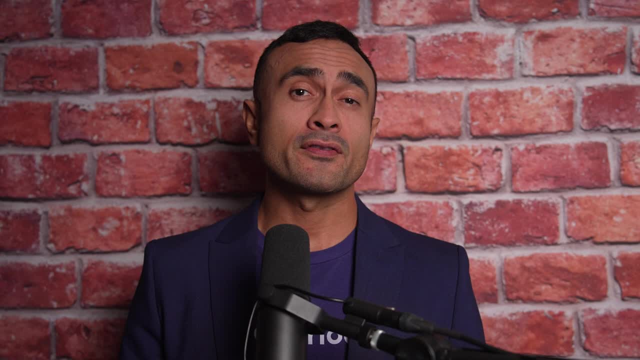 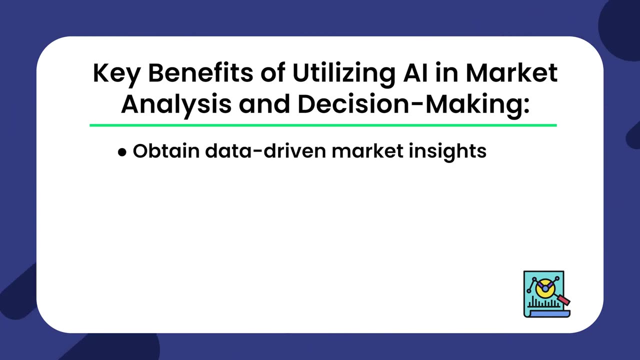 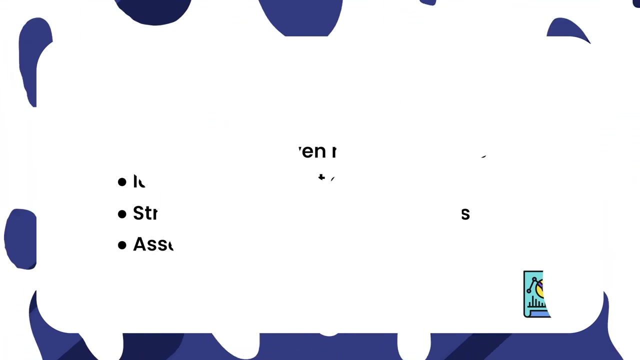 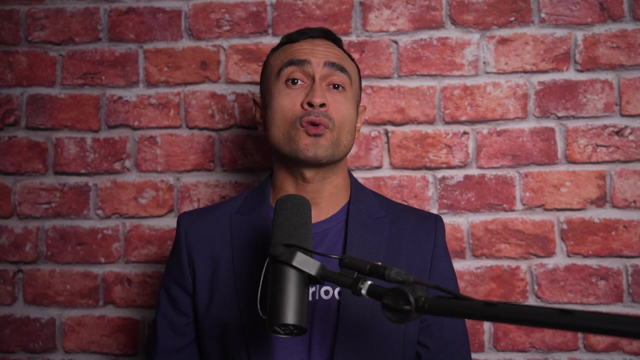 and maximizing your investment opportunities. Here are the key benefits of utilizing AI in market analysis and decision making: Obtain data-driven market insights, Identify investment opportunities, Strategically price your properties, Assess and mitigate risk. Workflow automation for operational efficiency. Artificial intelligence is all about automating tasks, and it's true for real estate as well. 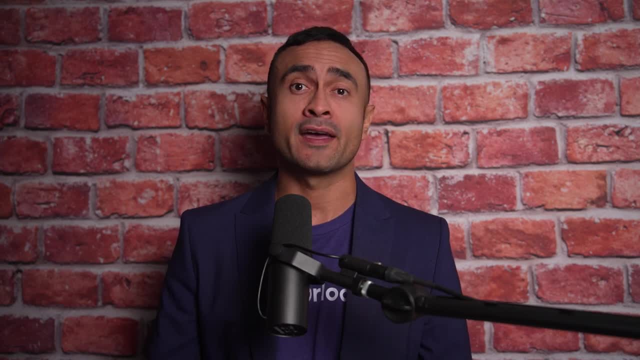 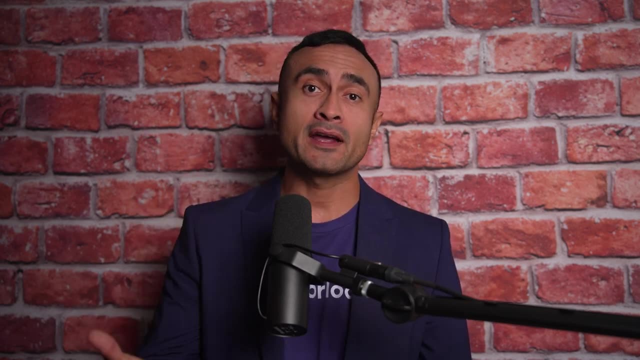 AI systems save time and resources for property managers and others in real estate by handling repetitive tasks like rent collection, maintenance requests, reminders and much more. This benefits not only property management companies, but also owners, investors and other real estate companies. 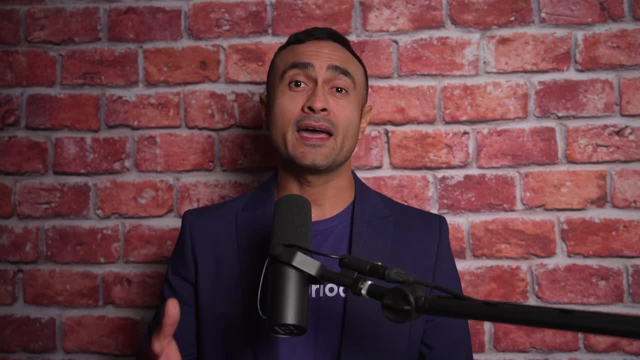 The AI-powered fraud detection and decision-making system is an essential part of the real estate market. AI automation also reduces the risk of errors that can happen with manual processes. By using AI tools or property management software, you can save time and focus on growing your 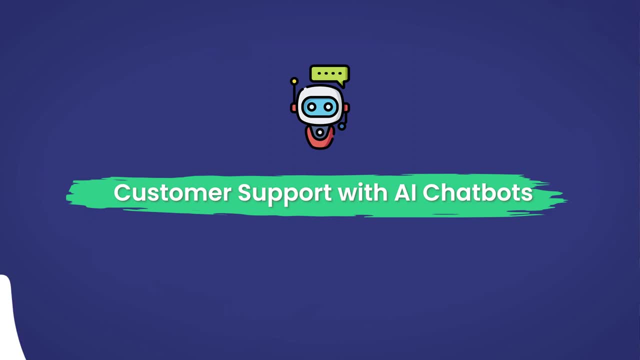 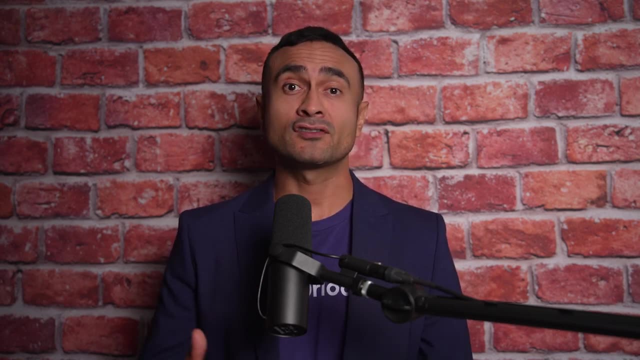 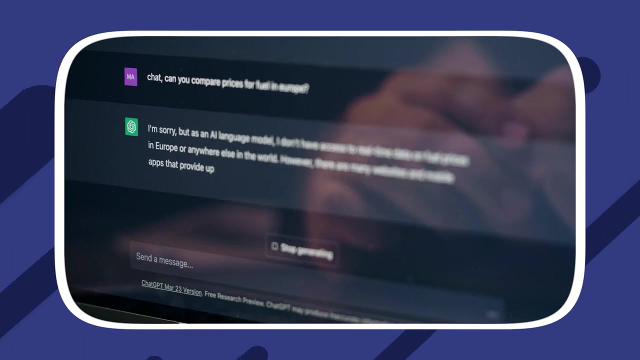 business Customer Support with AI Chatbots. Elevating customer support and service is another one of the ways AI in real estate is a powerful tool Based on deep learning technology. AI assistants like chatbots have given property managers managers and easy means to deliver prompt, personalized assistance to tenants. 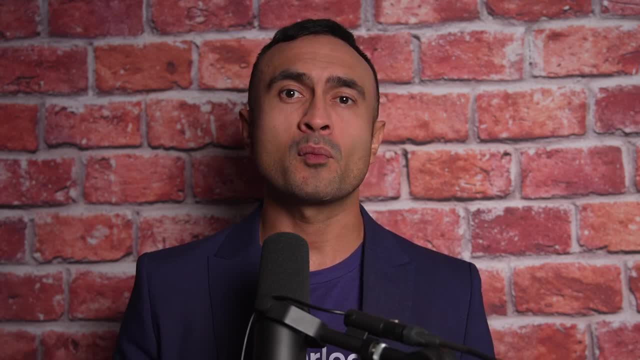 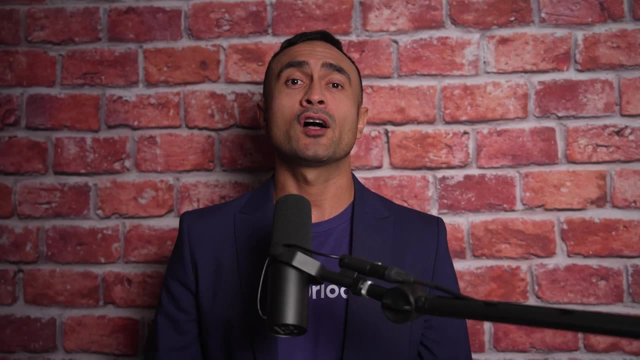 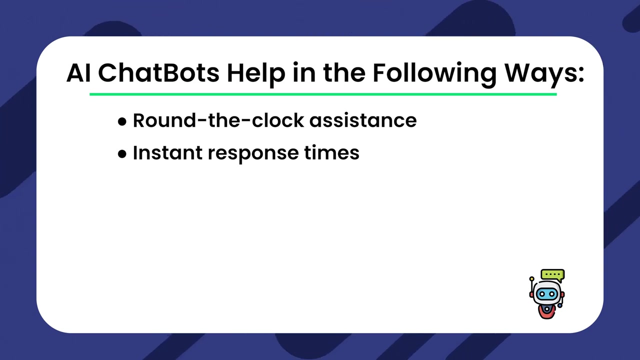 This mitigates the need for some human interaction, so that more processes are automated before reaching you. Among other benefits, AI chatbots and similar virtual assistants help owners and property management companies in the following ways: Round-the-clock assistance, Instant response times, Scalability and efficiency. 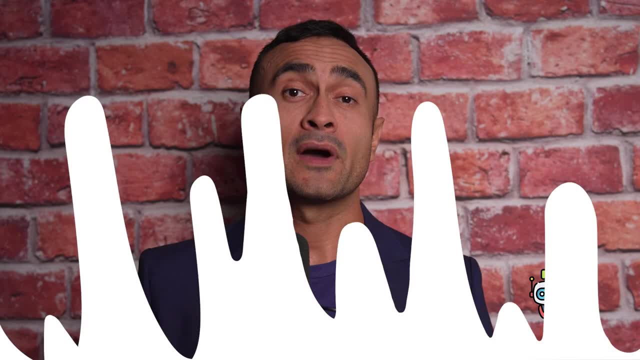 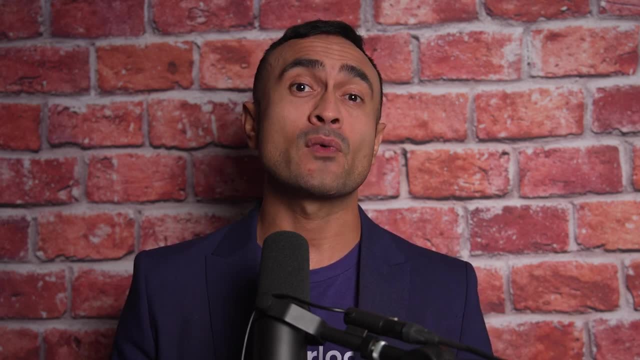 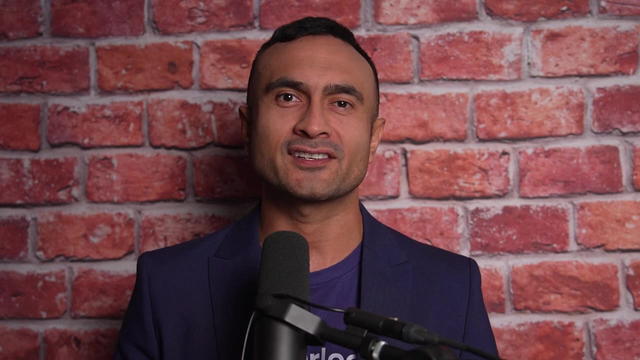 Reduced human error, Data collection and insights. By implementing AI, chatbots and customer support, property managers can deliver efficient, personalized and round-the-clock assistance to tenants, fostering stronger relationships and improving overall tenant satisfaction. All right, so let's wrap it up. 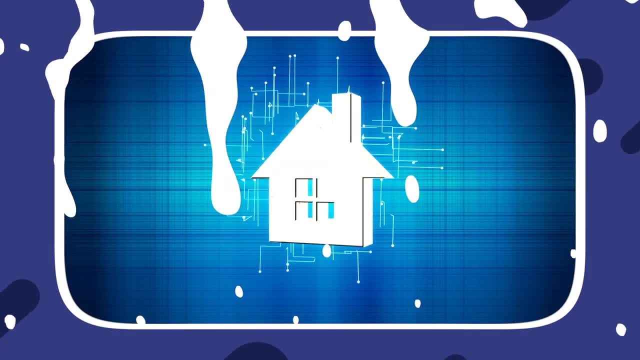 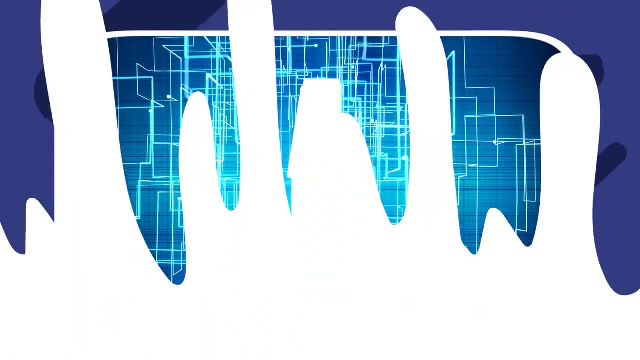 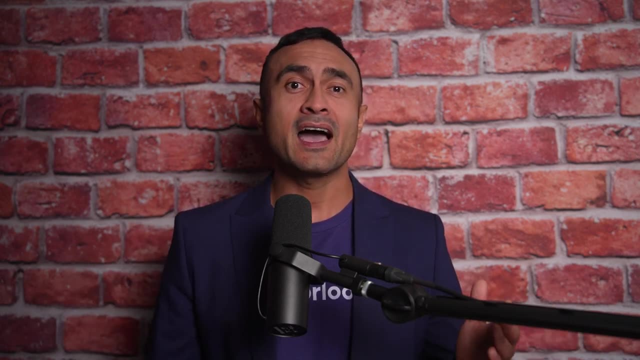 The integration of artificial intelligence applications in the real estate sector, and particularly property management, is revolutionizing the way real estate assets are managed: From automated property valuation To Introduction, intelligent lease management and workflow automation, AI in real estate is reshaping the industry.